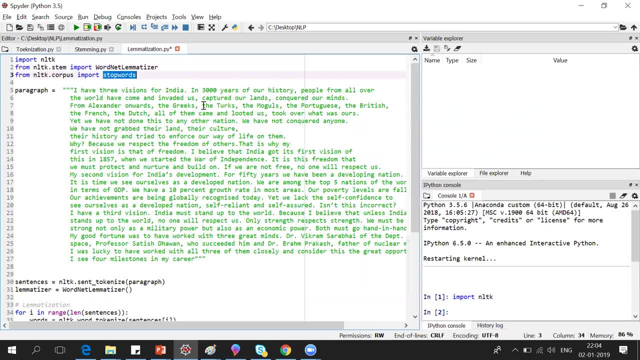 Stop words. is the library that is responsible for removing some of the words over here, like of. is the, that to and the. So these all words does not make a meaningful or does not play a better role when we are doing sentiment analysis. 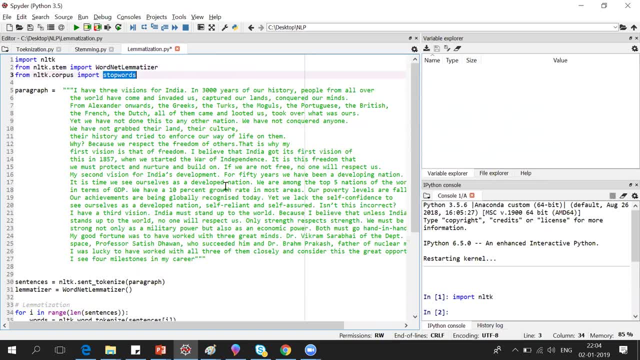 Because sentiment analysis usually happens on positive and negative words. right, If you find a positive word in a particular sentence, then we can, we can think, we can guess. at least it is a positive or a negative sentence. So this kind of words that we have like and the of the all this kind of us, all these, 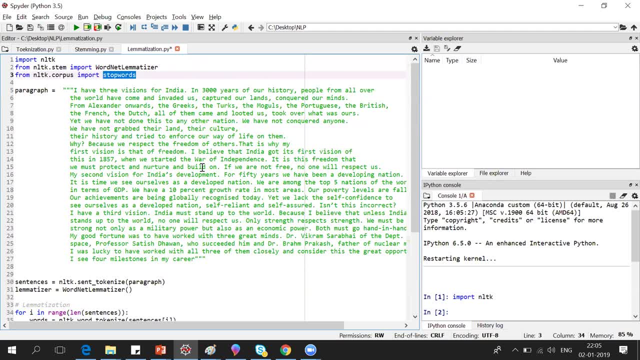 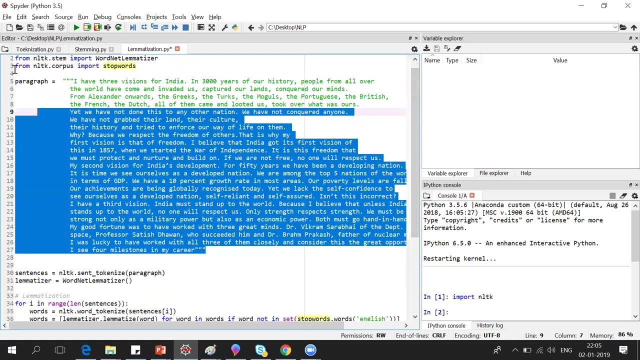 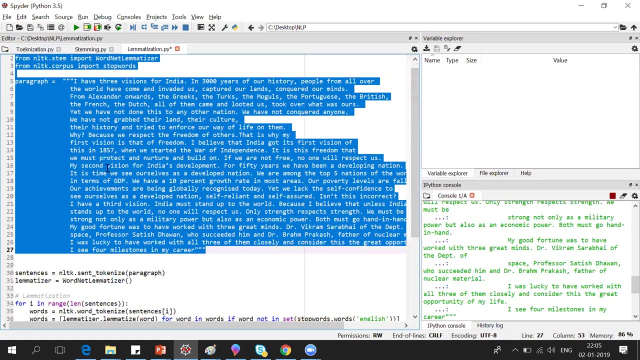 words. They are going to be removed by using the stop words which we have already discussed in our previous video. right now, Going forward Again, my first step is I'm going to first of all import and execute this three lines. that is, importing the library, WordNet lemmatizer. importing the library, that is stop words. 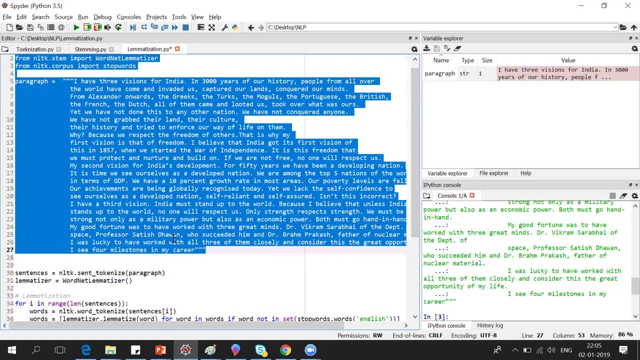 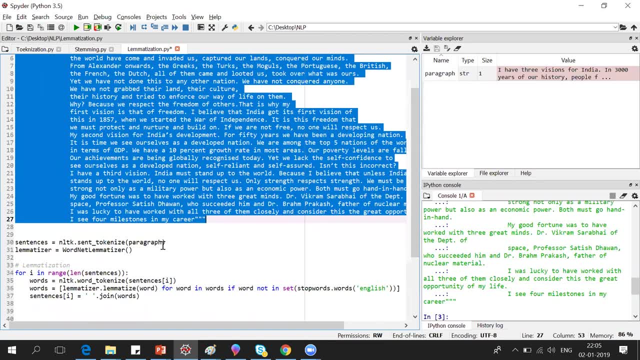 And you know the variable that is created. that is paragraph which is having my complete paragraph. Now you can see that the variable is created in the right hand side. The next thing that I'm going to do is that I am going to convert this. 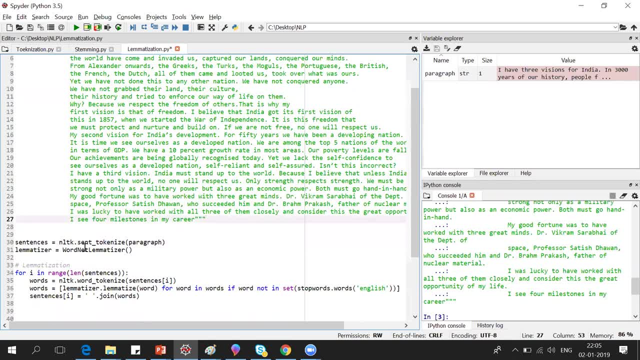 Whole paragraph into sentences, right? So once we convert this whole paragraph into sentences- and how can we do that- we'll be using a function that is present inside NLTK, which is called as sent underscore tokenize. So once I execute this, you can see that I'll I'll convert this whole paragraph into sentences. 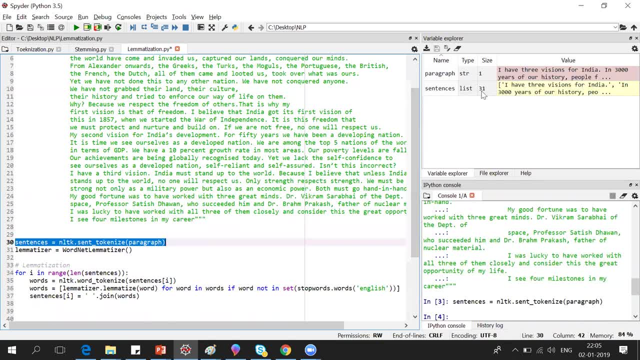 And let us see how many different sentences we'll be getting. So we are getting around 31 sentences. So these are all my sentences Right Now. The next step is that what we will do is that we will import the library that was import. 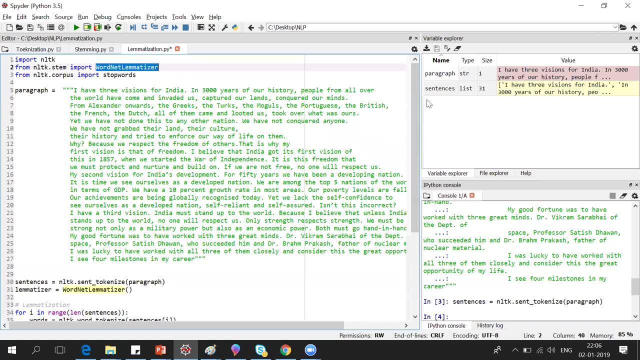 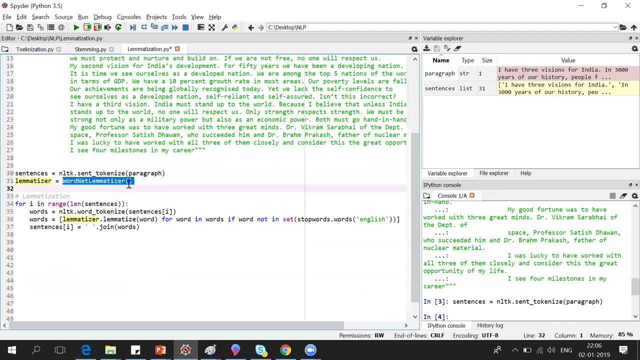 for lemmatization imported. for the lemmatization that is WordNet lemmatizer, I'm going to create an object for this. So here is my lemmatizer object that is created from this particular WordNet lemmatizer. 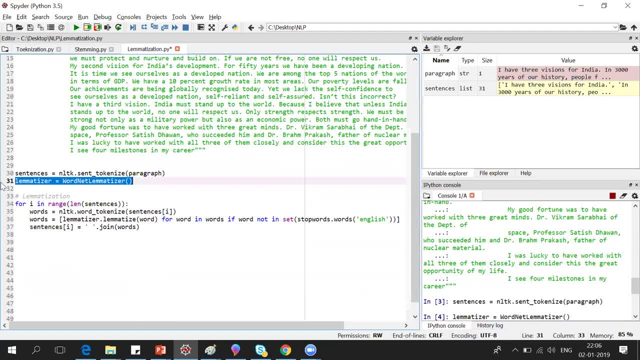 So let me just execute this and guys responsible. This object will be responsible for doing the lemmatization function. Okay, Fine, This has got executed perfectly. Now Let's add a new paragraph in here. Let's call this one: 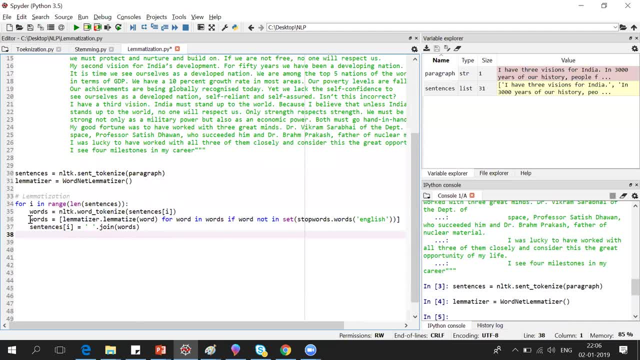 So I'm going to add a new paragraph. So if I click on an image, I'm going to add an image on this section and I'm going to say, Oh, there is a lot of little letters that I have and all the other letters are. 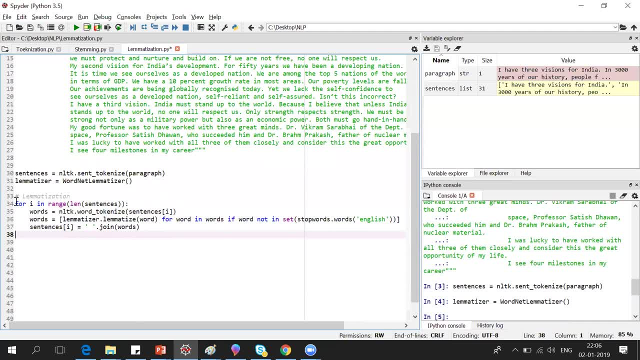 looking pretty on it, Like the lines are moving in the right direction. These lines are moving in the wrong direction, So I'm going to keep them in the same direction. That's a small difference. So first of all, I'll go and put a for loop in the list of sentences that I have. 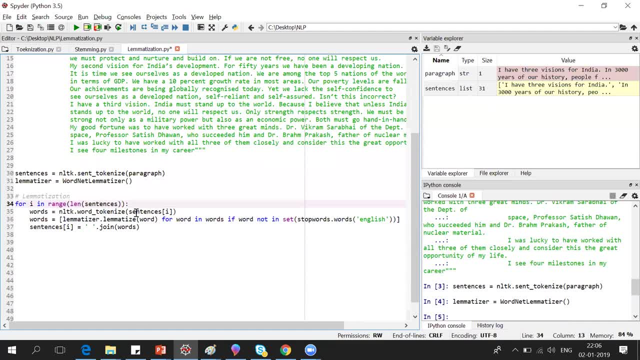 So I'm using the range of length of sentences. Okay, So if I execute length of sentences, you can see that if I execute the length of sentences over here, I'll be getting a value as 31.. I've got the value is 31.. 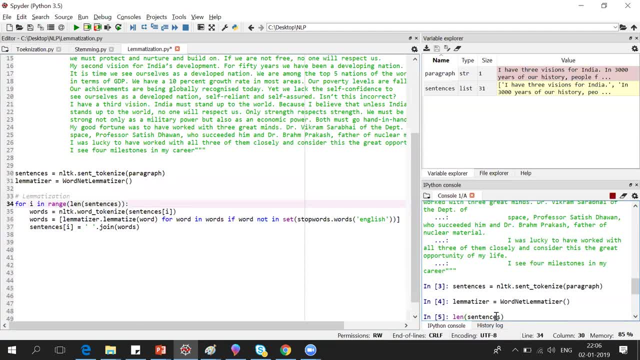 if I execute the length of sentences over here, I'll be getting a value as 31. I've got the value as 31. so when I write range of 31, that basically makes a range of 0 to 31. so 31 times this loop will run, then the first loop. what it is going to do is that it's going 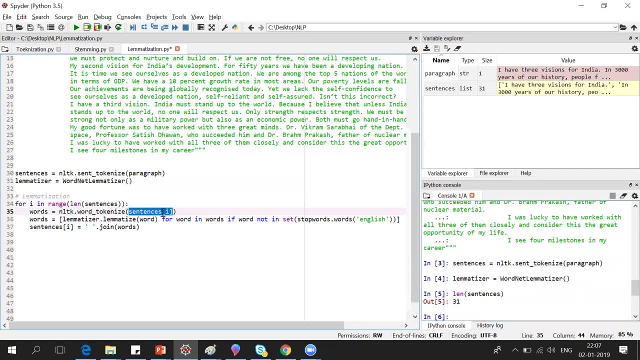 to take that sentence, the first sentence, and then it is going to convert into words. how it is going to convert into words? by using the nltkword underscore tokenize function. so once we execute this, our words is actually created. a lot of words will be created here, right so from the first. 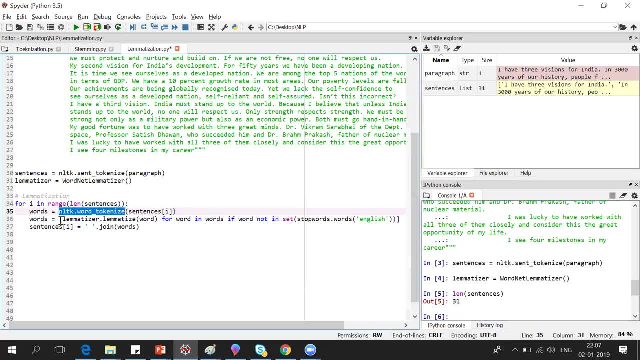 sentence, for each and every sentences, we'll be creating the word, then we'll be applying a list: comprehension. this is the most important sentence, which is almost like stemming. only one thing: there will be a difference for word in words if that word is not present in stop word, which is 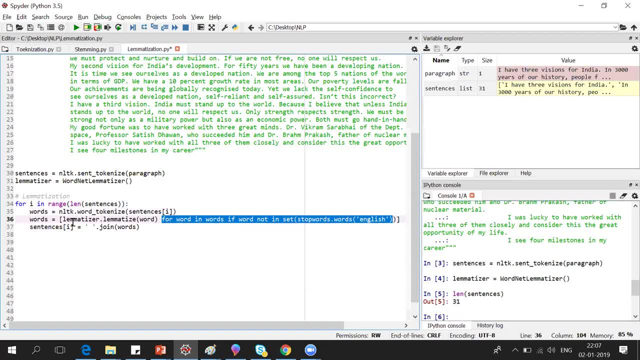 in English language, I'm going to take that word, and I'm going to take that word and I'm going to write something like lemmatizer dot. lemmatize. lemmatize is the function which is responsible for doing the lemmatization process, and inside that I'm going to provide that word. if it is not. 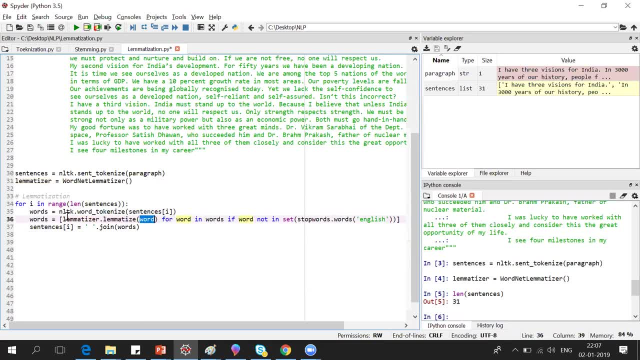 present in the stop words. so after I do that I'll be getting a list of words in this particular words- variable- and after that I take that words, I join it and I convert back that that into sentences. so this sentences will actually consider the number of words that are present in the stop words. 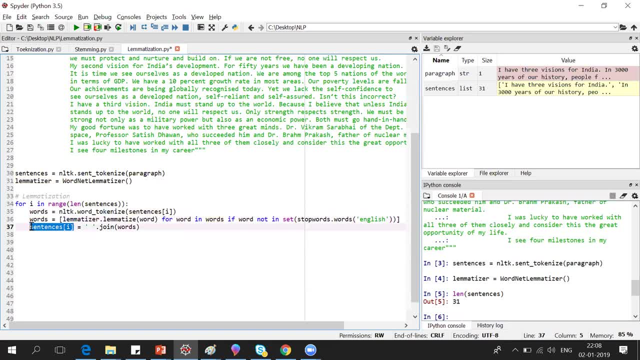 and then I'm going to do the lemmatization, so it will be consisting of all the lemmatized words in this particular sentences, and this will happen thirty one times. that is all the basically. how many length of the sentences are there with respect to this list? they are on 31, 31 times.